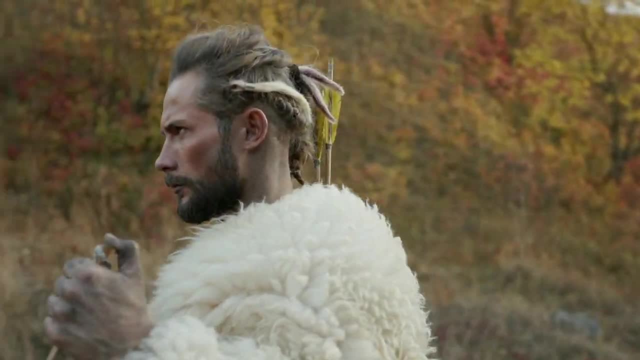 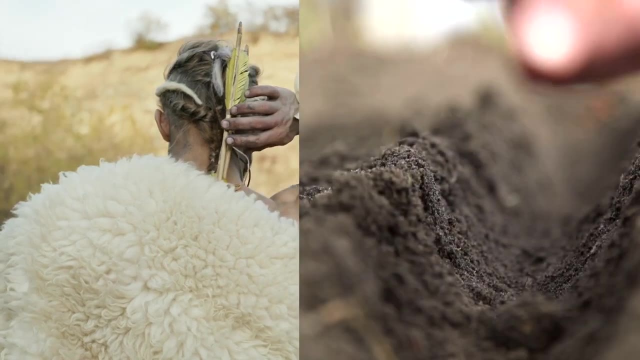 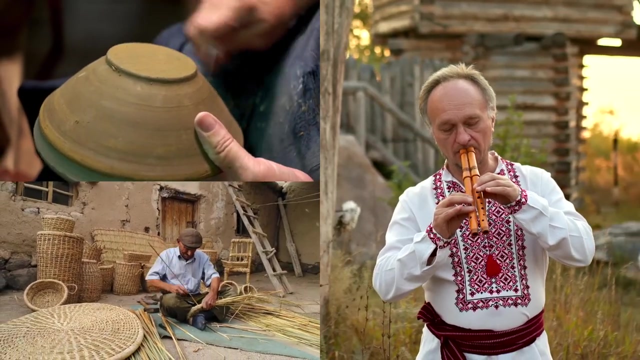 Life was good. According to historians, it took humans around two and a half billion years, give or take a few- to move from hunters and gatherers to farmers and herders as primary methods to gather food. Specialization occurred soon thereafter in ancient cultural. 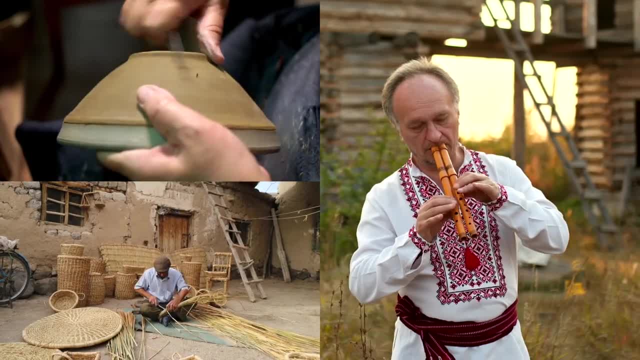 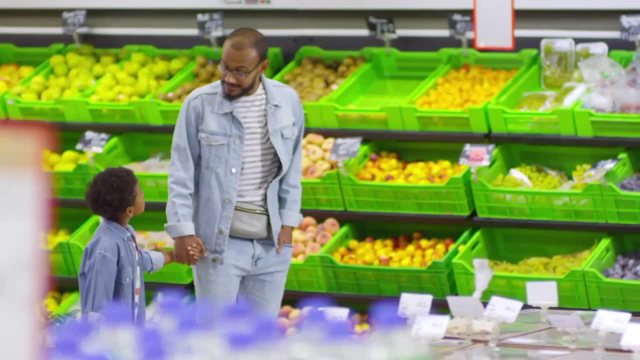 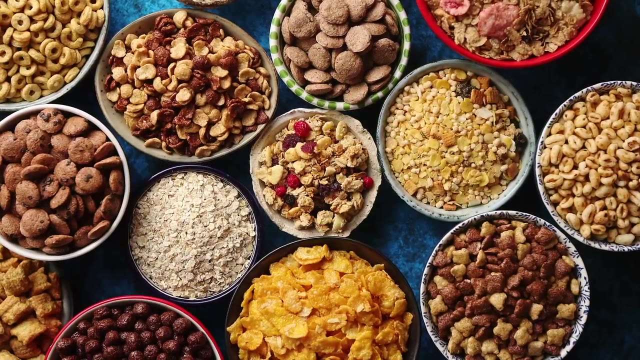 hearths like Mesopotamia, Egypt, India and China, allowing some individuals to trade for food in markets rather than growing it themselves. And, of course, this all leads us to today's trips to Kroger and Walmart to scan the breakfast aisle and pick up one of the 2,000 series of 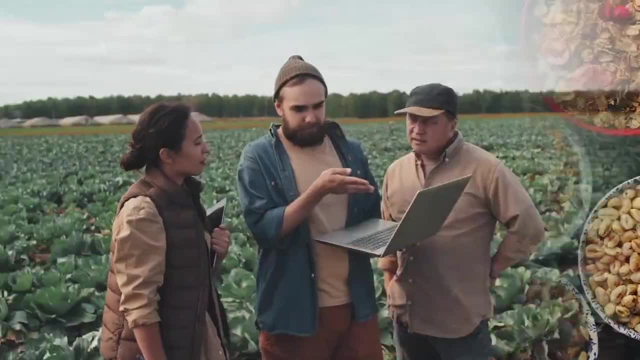 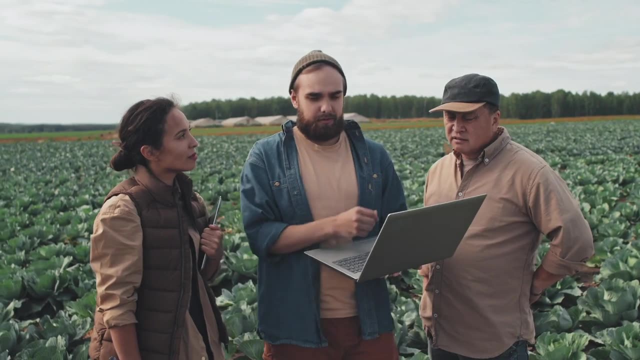 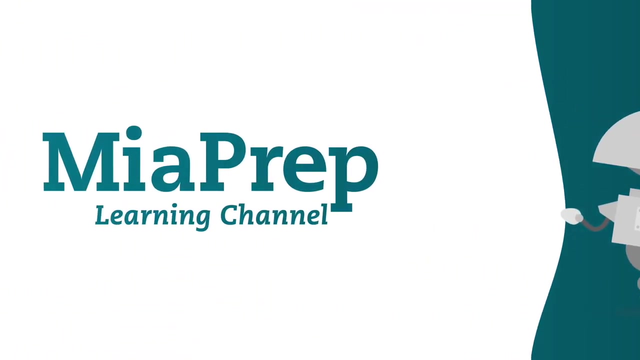 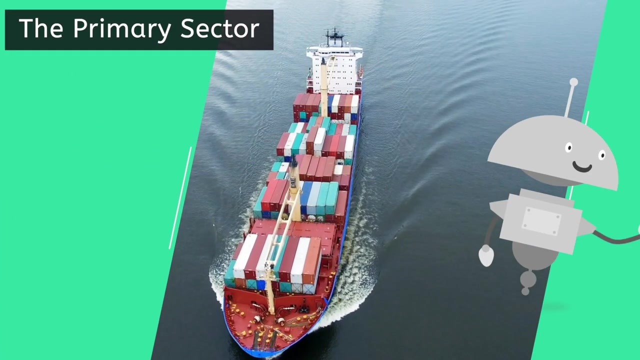 materials that you've seen ads for on TV. We've come a long way in the last 12,000 years, and today we'll uncover how goods like food, furniture and ideas end up within our reach, Ready explorers. So 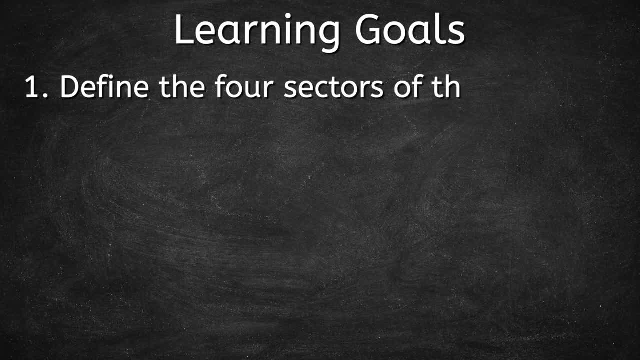 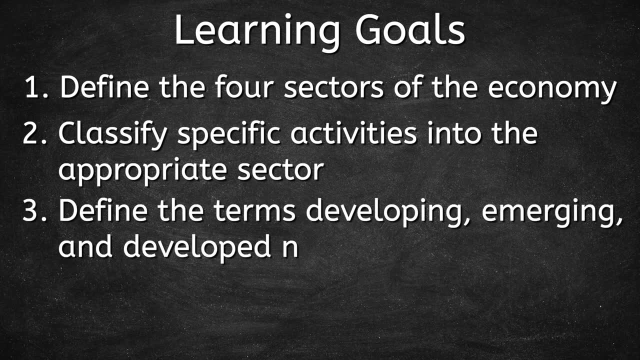 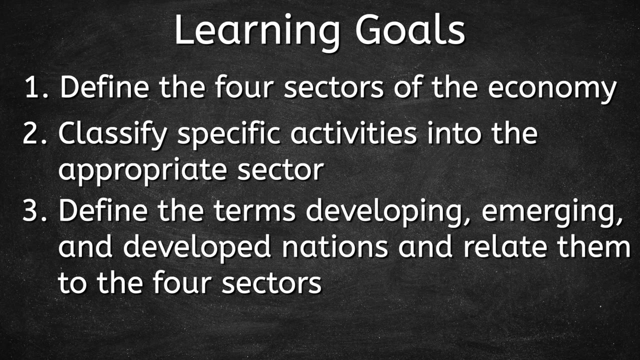 our learning goals for today's trip are: to define the four sectors of the global economy, to classify specific activities into the appropriate sector. to define the terms developing, emerging and developed nations and relate them to the sectors of the economy. All economic activity is grouped into four sectors: primary, secondary. 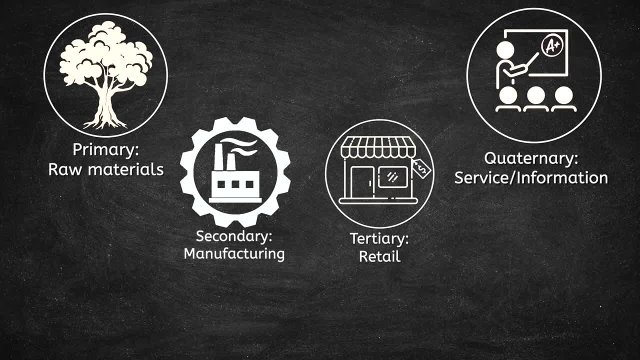 tertiary and quaternary. Of course, fancy words for first, second, third and fourth don't sound very creative, but it has to do with the fact that we're in the middle of a world where we're looking at the past, past, present and future. So let's start with the first sector of the world. 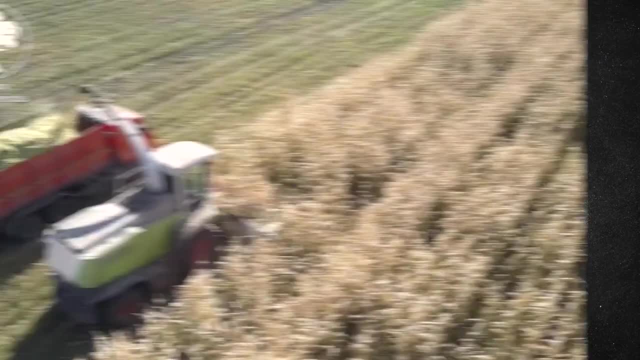 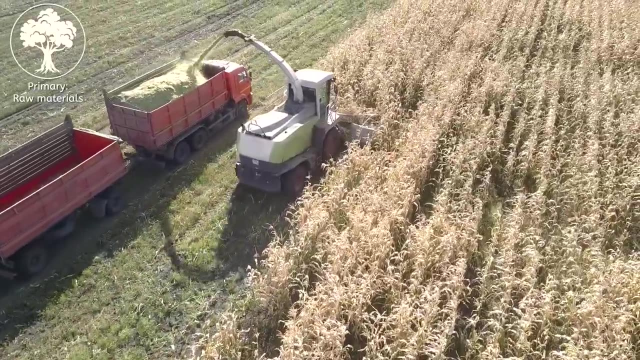 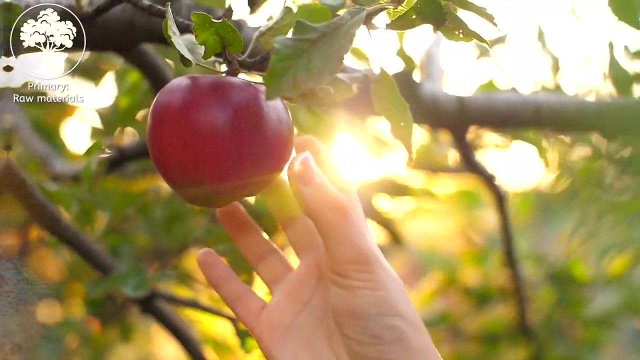 and, first and foremost, let's look at our knowledge of natural resources. Let's start with the primary sector. Primary economic activity refers to the extraction of raw materials from the earth. Farming is the most important and most prevalent primary economic activity, Whether it's growing crops, fungi or livestock on huge commercial farms. 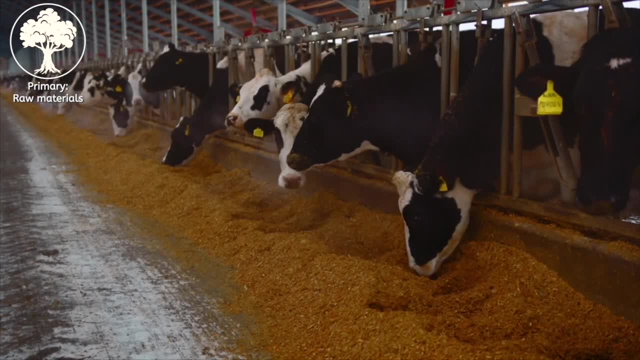 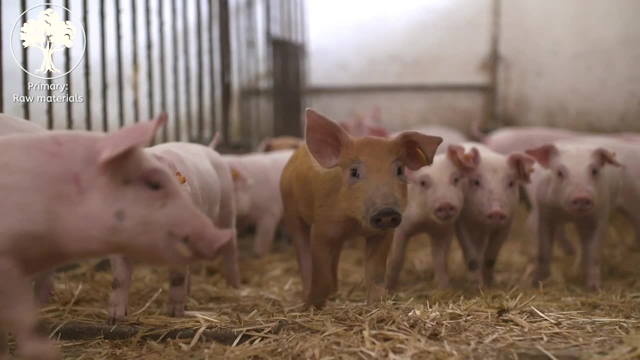 or in subsistence gardens. all of it is considered primary economic activity, But, as you learned in our natural resources series, we're going to be looking at the most important and most prevalent lesson. plants and animals aren't the only natural resources that humans extract from the environment. can you come up with another example of primary 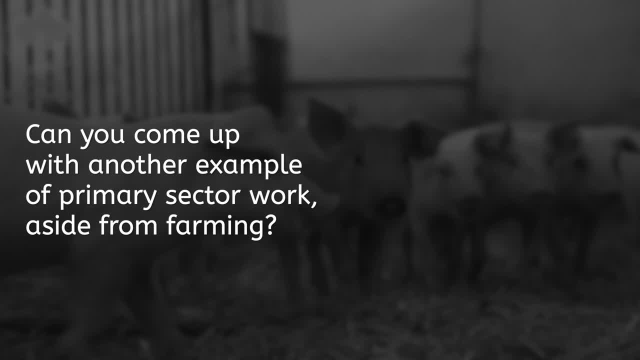 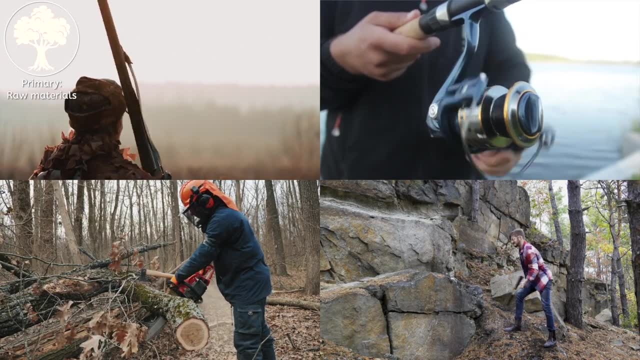 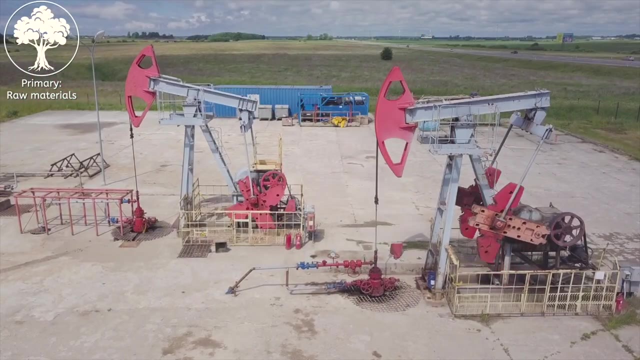 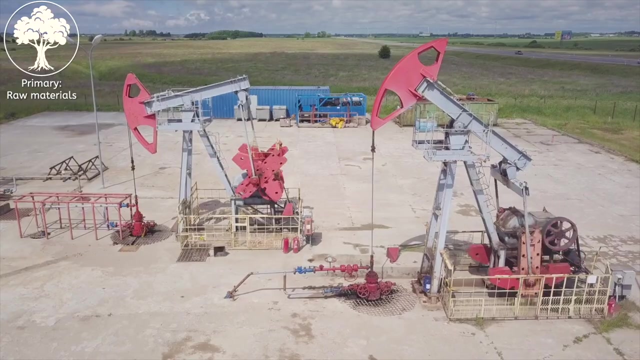 sector work aside from farming. pause the video and answer in your lesson guide. that's right. other primary economic activities include hunting, fishing, forestry and mining. all of these activities involve taking resources from the earth. whether those resources are crops, animals, minerals, metal, lumber, renewable or non-renewable, each one features humans harvesting raw materials. 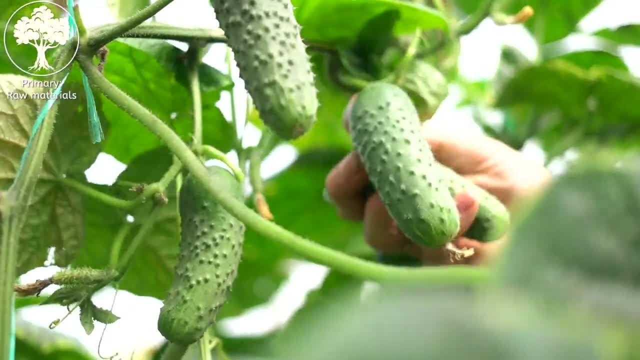 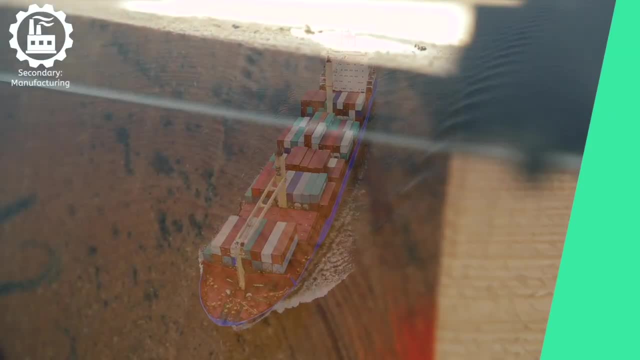 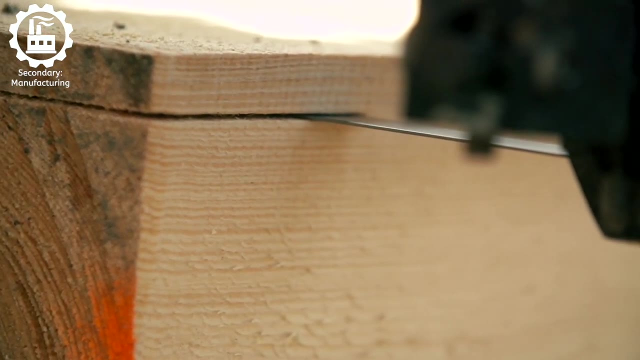 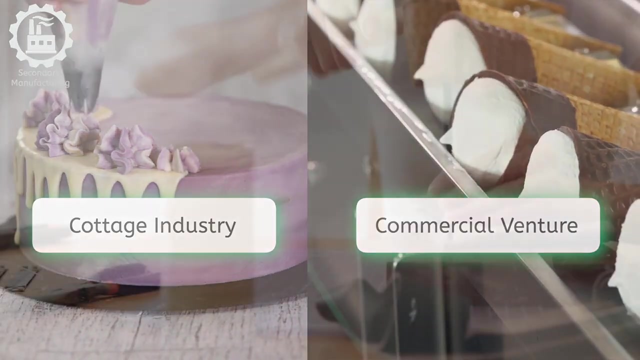 from the lithosphere, hydrosphere, atmosphere and biosphere. secondary economic activity is the processing of the raw materials produced in the primary sector. many people call it the manufacturing sector. it includes both cottage industry and commercial ventures. cottage industries are often home-based and always small-scale. in ancient civilizations. 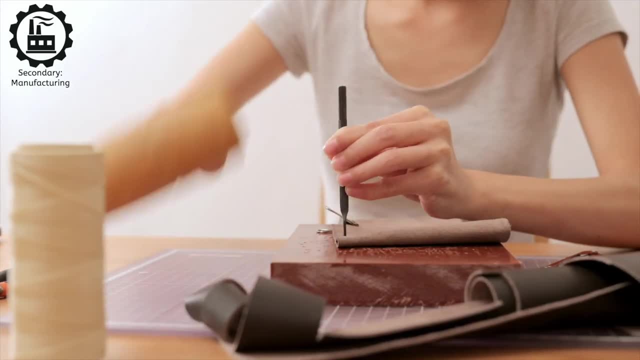 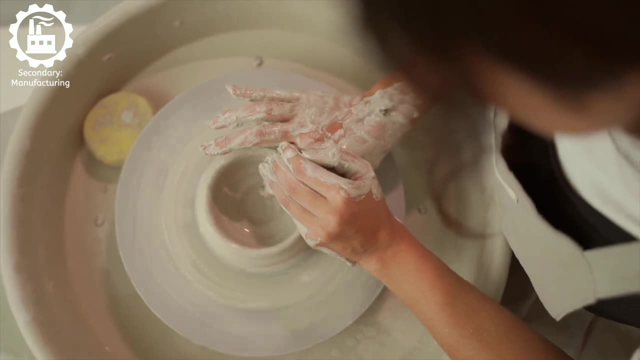 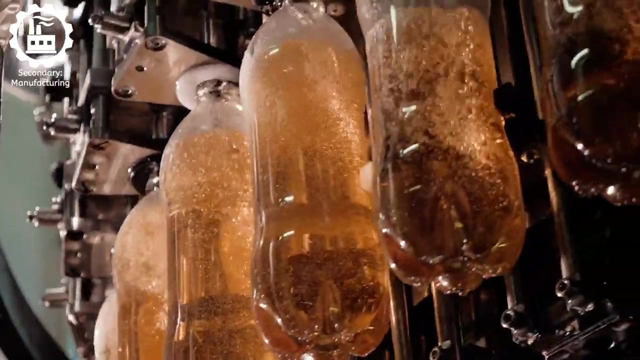 those included someone who made pottery. we've drugs created clothing or ground corn into meal. if you've ever bought something on etsy, it's probably a cottage industry product commercial industries are also included in secondary economic activity and are much more common today: large-scale businesses that employ many people and mass-produce identical. 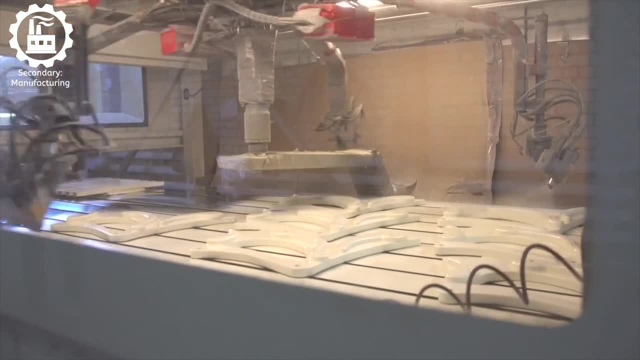 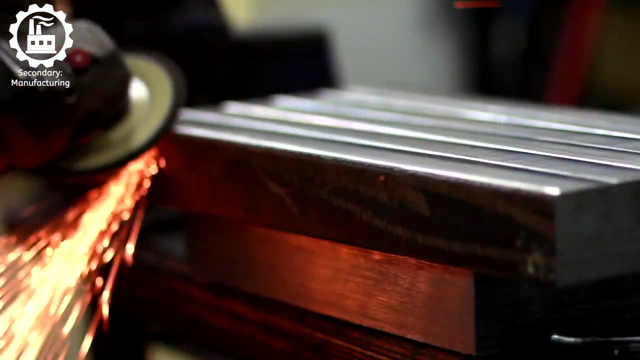 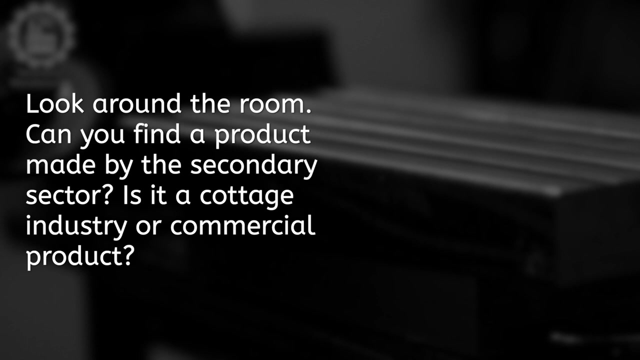 products. Examples include a furniture factory that turns wood into tables and chairs, or perhaps one that turns iron ore into steel to be used in home appliances. Take a second to look around the room. Can you find a product made by the secondary sector? Is it a cottage industry or commercial product? Jot down. 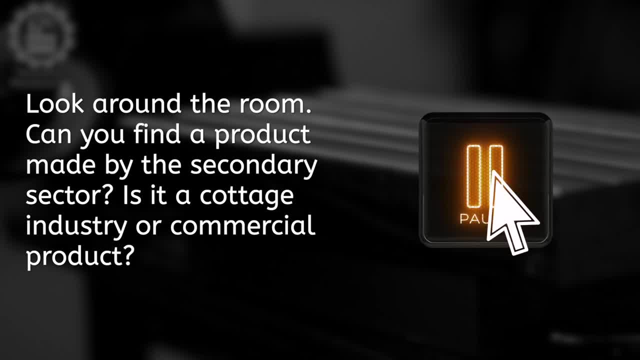 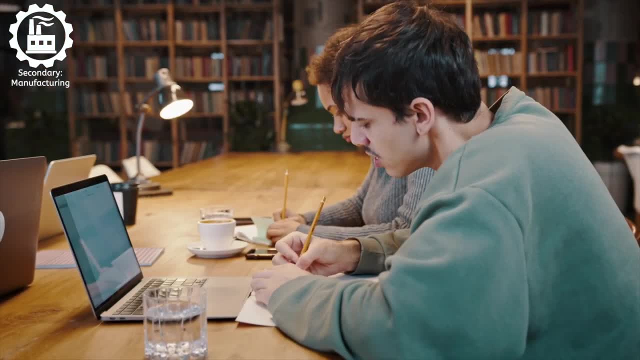 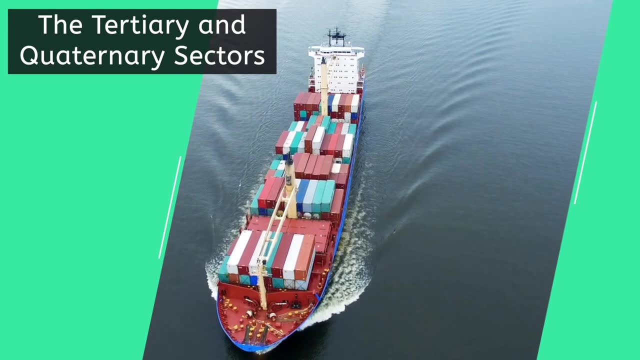 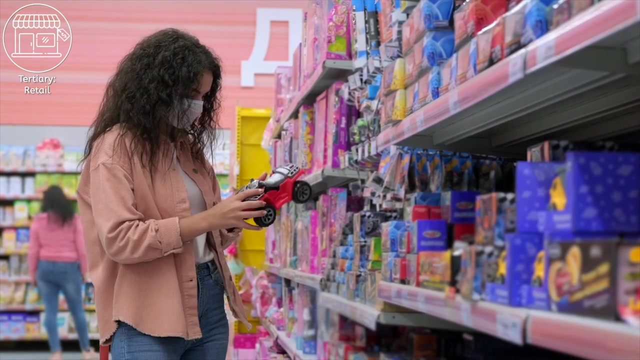 a response. in your PDF Maybe you said the table or desk you're using to work on your lesson guide is a secondary sector product and if your family got it from a big furniture store, it's probably a commercial product. Speaking of a big store, that's a great example of a tertiary sector activity. 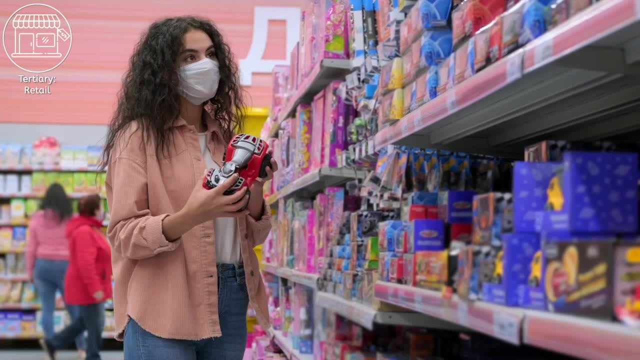 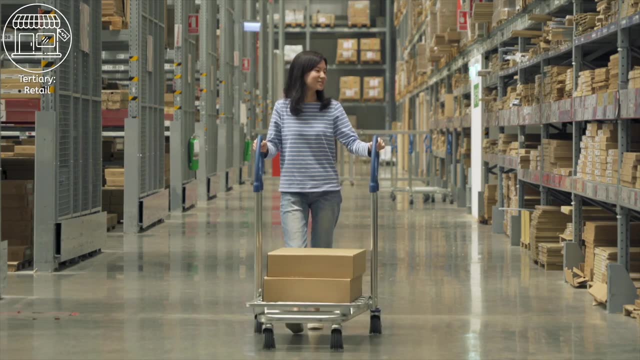 This sector is nicknamed the retail sector. Tertiary sector is a category of activity that involves a large number of people. Tertiary activity is the sale of manufactured goods. Okay, it's the sale of raw materials too, if you want to get picky, but most retail stores sell. 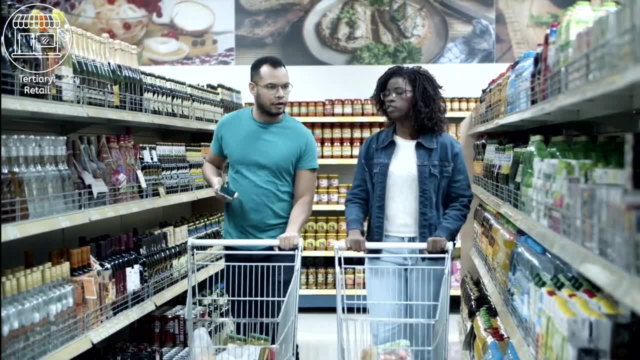 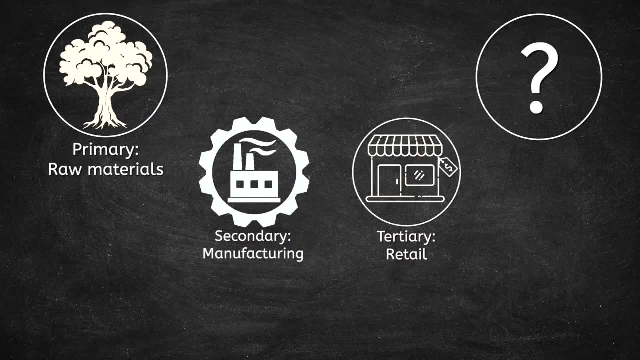 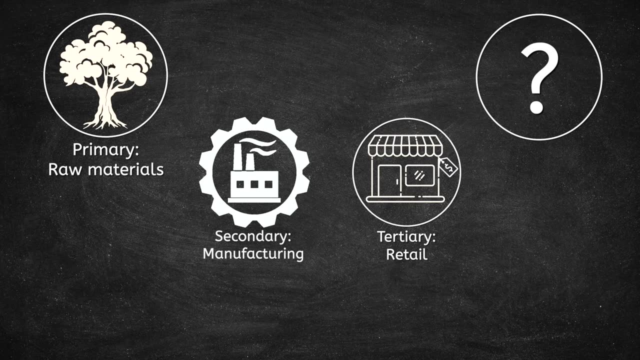 manufactured goods nowadays. So when you head to the grocery store to get that tasty cereal, you'd be involved in tertiary activity From here. the sectors are different depending on who you ask. Some people say there are only three sectors and that anything that isn't a primary or secondary sector activity 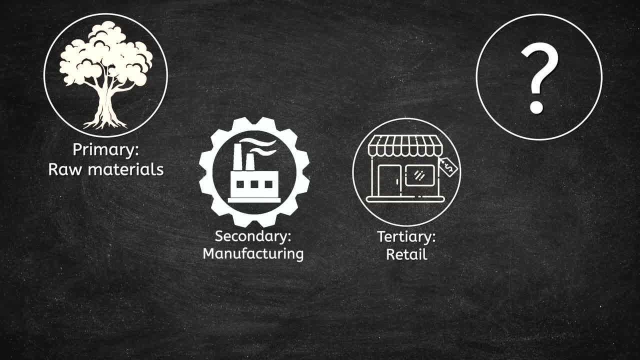 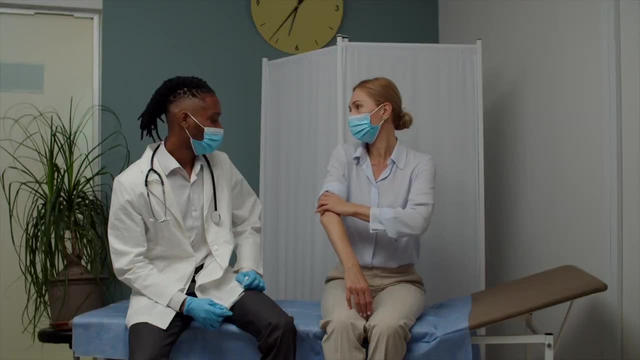 belongs in the tertiary sector. But the numbering system is based on the relationship to natural resources, right? So what if someone's job has nothing to do with natural resources? What about a teacher like me, an explorer like John, a sensei, a business consultant or a doctor? 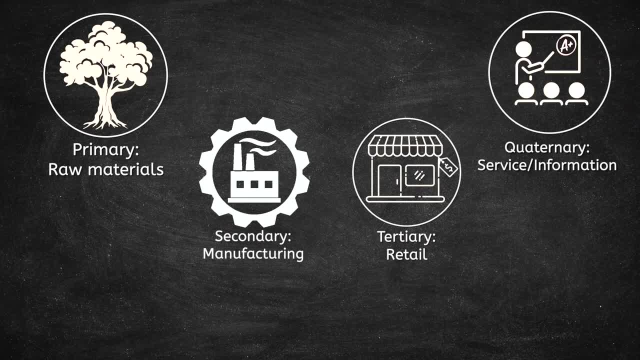 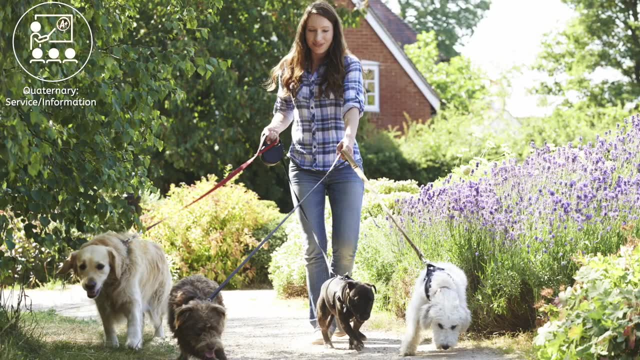 This is where the quaternary sector comes in. For some, this is called the service sector. That would mean that it involves completing a task like dog walking for someone instead of offering a tangible product. For others, this is called the information sector, which means that it 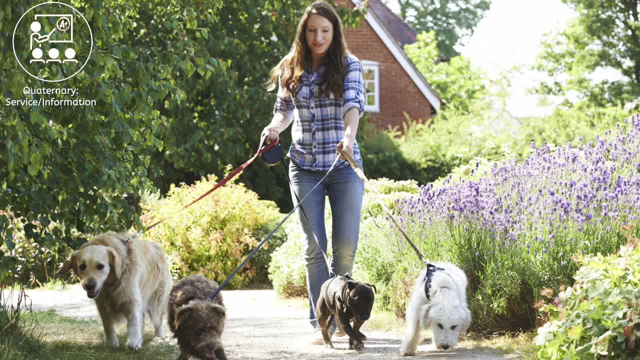 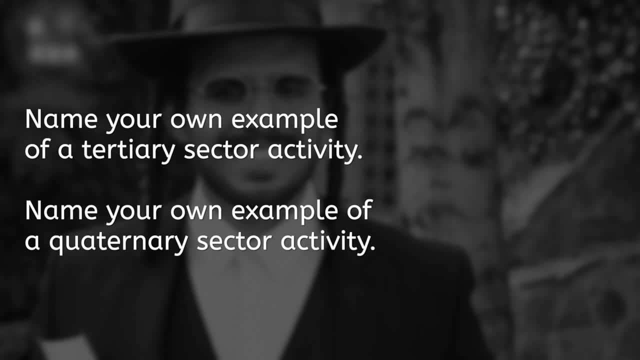 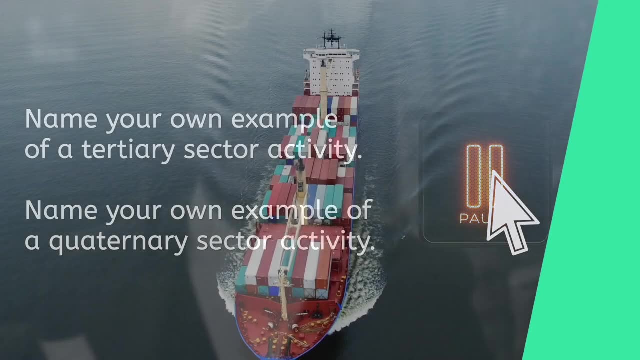 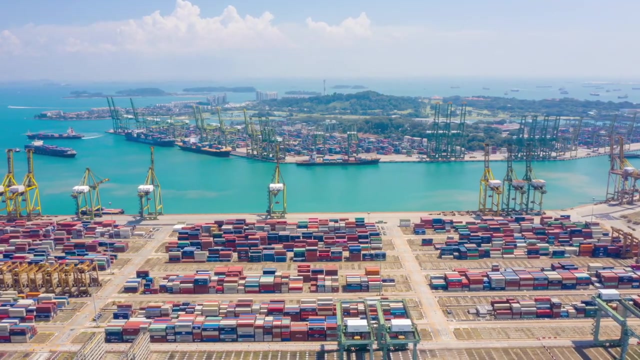 involves the transmission of intangible products and services. A rabbi would be a good example of this. Take a minute to come up with your own example of a tertiary sector activity and quaternary sector activity in your lesson guide. Understanding these sectors will help us describe the. 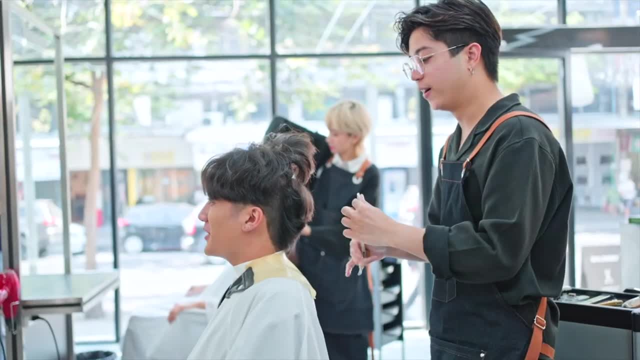 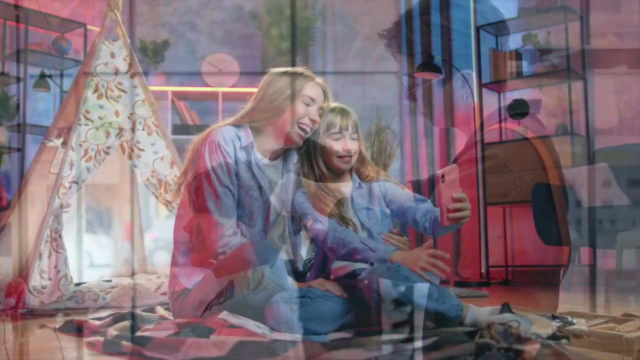 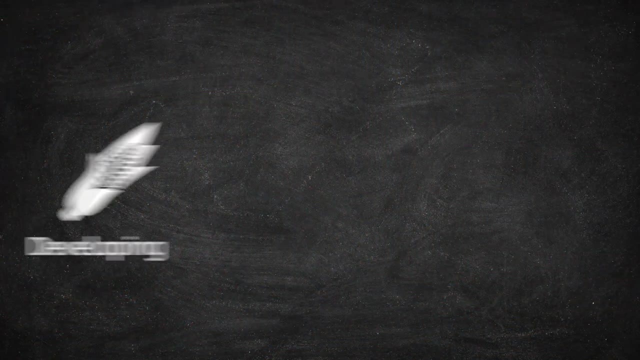 economic development of countries we visit this year. Knowing which sector people work in helps us to understand the standard of living and average income of people within a society, which are indicators of their access to international products and the influence they have around the world. In this framework, all countries 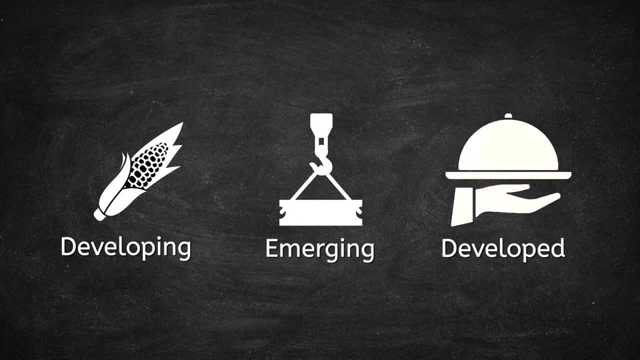 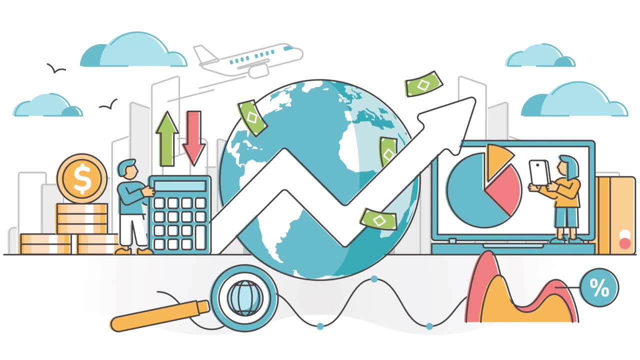 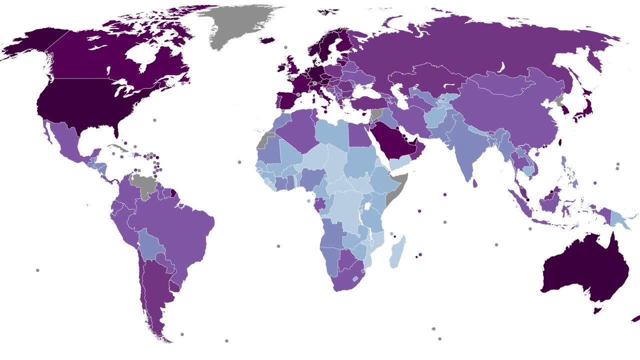 are sorted into three categories – developing, emerging and developed. There are two measures commonly used to determine which category a country belongs in For the. The first is called Gross Domestic Product, or GDP. This is a measure of what people produce in a country. 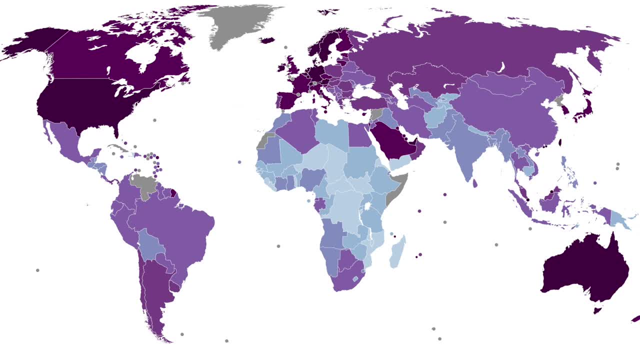 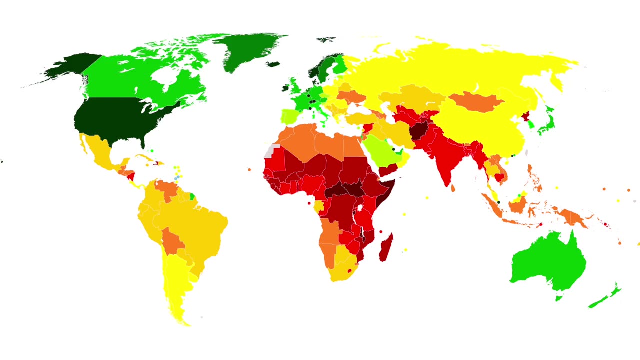 This map shows GDP per capita. The data shows that US, German and Australian citizens are very productive, while the people of Central Africa are less productive in terms of economic output. Another litmus test is per capita income, a measure of how much money people earn.